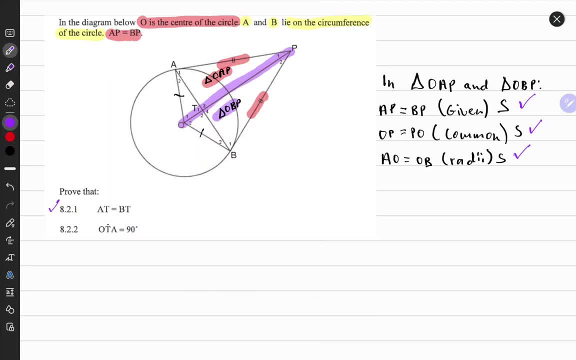 So, through the condition side side side, we can say that these two triangles are without a doubt congruent And because of congruency, the angles across the equal sides, O1 is across this side, across that side, we can say that, therefore, angle O1 is equal to angle O2. 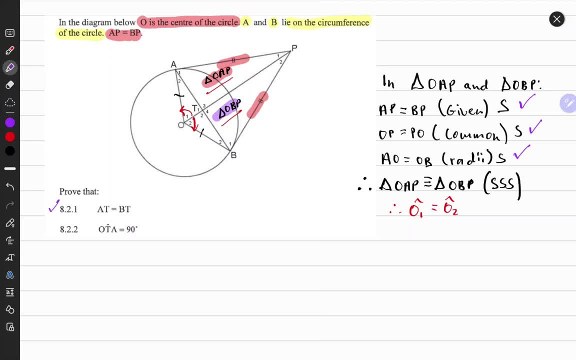 so let's focus our attention to the smaller triangles corresponding smaller triangles, that is, OAT and OBT, so that we can try and prove congruency in those triangles in order for us to show that these two sides are equal in length. so notice that in triangle OAT and OTB, this side here, OT, is equally long for both. 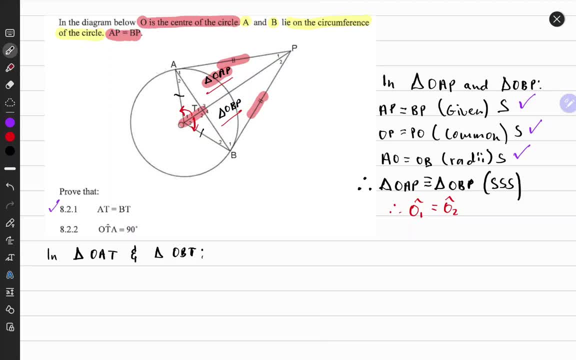 triangles. so that's why we can say that OAT and OTB are equal in length. so notice that in triangle OAT and OTB- this side here- OT is equally long for both triangles. so that's a common side. so that's worth noting. we can say that OT is equal to TO. 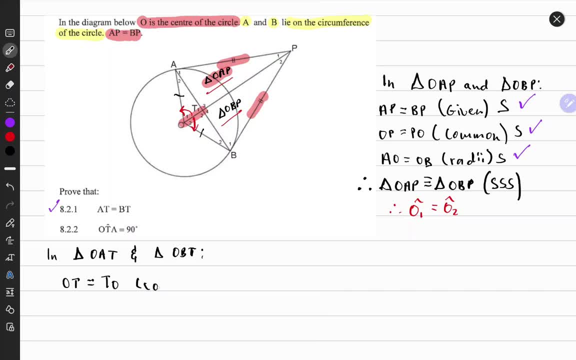 T? O. that's common, so we have a pair of corresponding sides. also, angle O1 is equals to O2, because we saw congruency of the bigger triangles equal to T? O and that's worth noting. So now we have a pair of corresponding angles and of course, side AO and side OB. 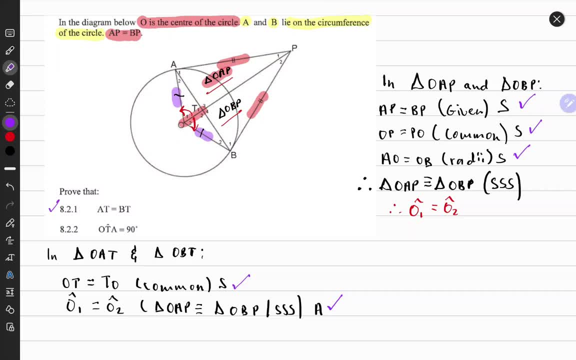 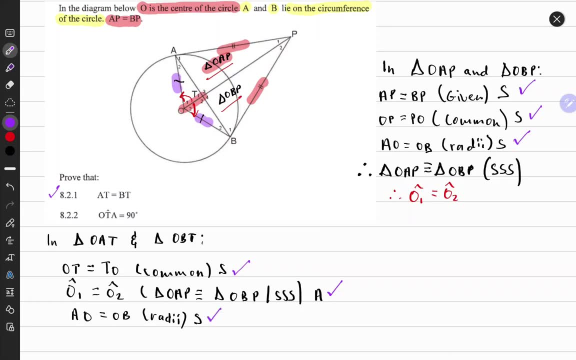 are equal in length because of radii, so it's worth noting that as well. So that's another pair of corresponding sides. so through the condition side, angle side, we can say that triangle OAT and triangle OBT are congruent, and because of congruency between those two,